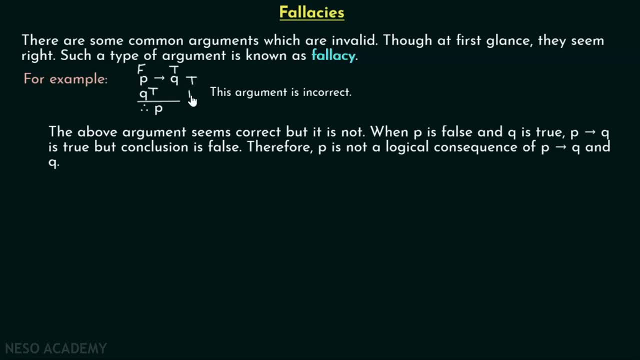 Here you can see that this Q is true. That means P implies Q is true And Q is true. But let me tell you that conclusion is false. So it is clear that our conclusion, that is, P, is false. Therefore, P is not a logical consequence of. P implies Q and Q. 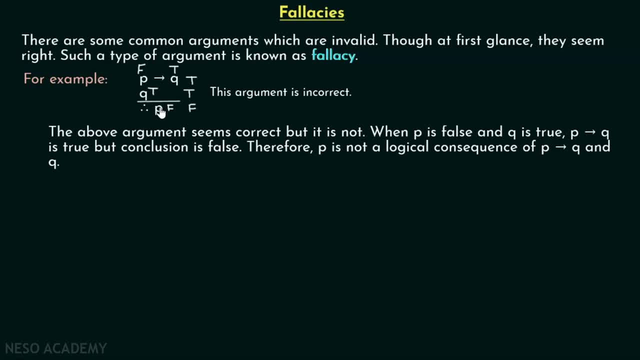 It is clear from this fact that P is not logical. consequence of P implies Q and Q. The above argument is called the fallacy of affirming the conclusion. It has given a name. It is so popular that it has given a name. the fallacy of affirming the conclusion. 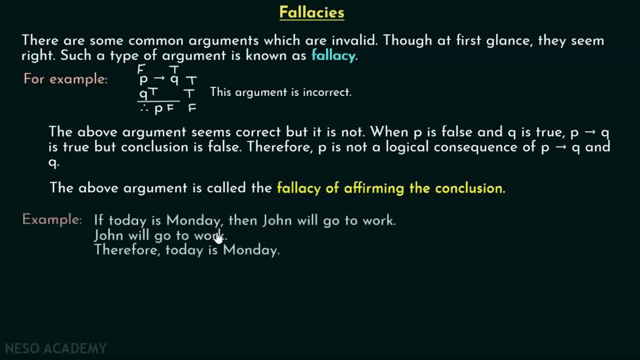 Let's see one example to cement this. If today is Monday, then John will go to work. John will go to work. therefore, today is Monday. It seems correct, right? But let's see this properly. Let P denotes today is Monday and Q denotes John will go to work, right? 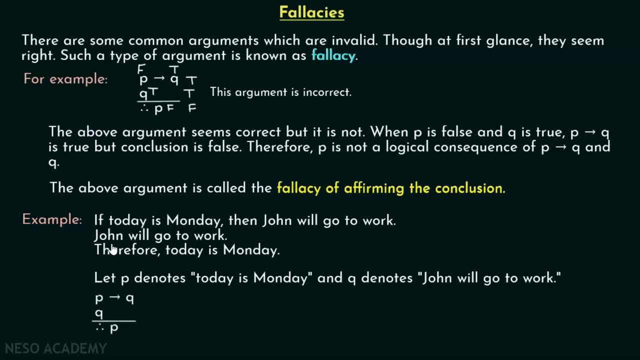 From the first premise we can write P implies Q right. And from the second premise we can write Q And the conclusion is: today is Monday, which is P right. So this is an argument- And you already know that this is fallacy- of affirming the conclusion. 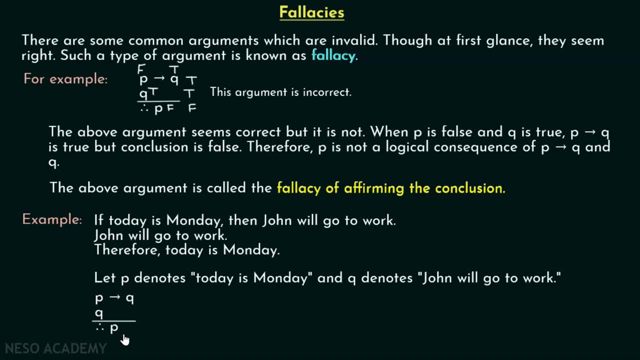 This argument seems valid, but this is not. This is a fallacy. Let's understand this, why? Here you can see that if today is Monday, then John will go to work. Understand this: If today is Monday, then John will definitely go to work, right. 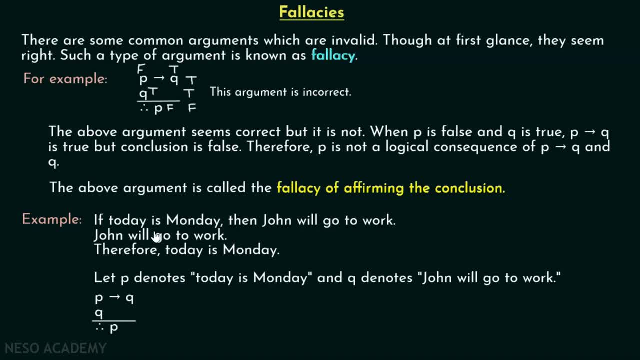 John will go to work. This is true. Can you say that today is Monday? Obviously not right. It doesn't mean that John will go to work. implies: today is Monday. Obviously this is not the case. But if today is Monday, then John will definitely go to work. 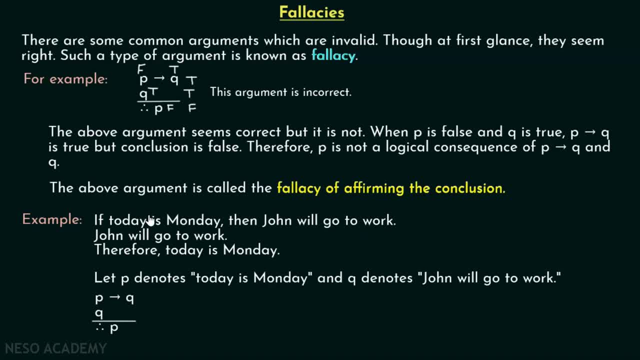 But the other side is not true. It may be possible that it could be true. It could be some other day, right? Therefore, today is Monday is not a logical consequence of these two premises? right Now, let's discuss one more popular fallacy. 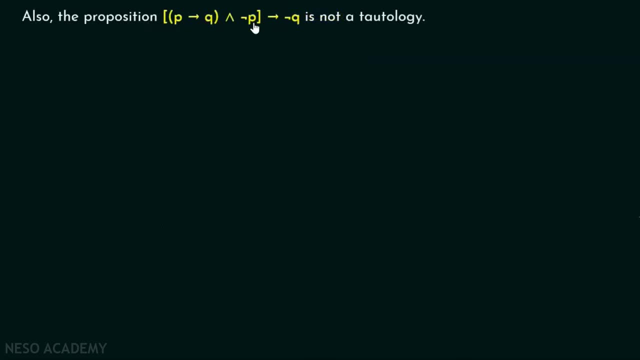 You can see over here. this preposition is not a tautology. P implies Q and not P implies not Q. It seems like this is modest Stalin's rule, but this is not Here. instead of not Q, you have not P. 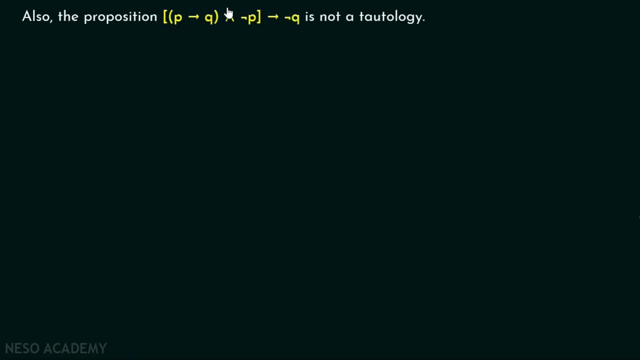 And here, instead of not P, you have not Q. This is not a tautology, Because when P is false and Q is true, let's say, when P is false and Q is true, then P implies Q is obviously true and not P is true but not Q is false, right? 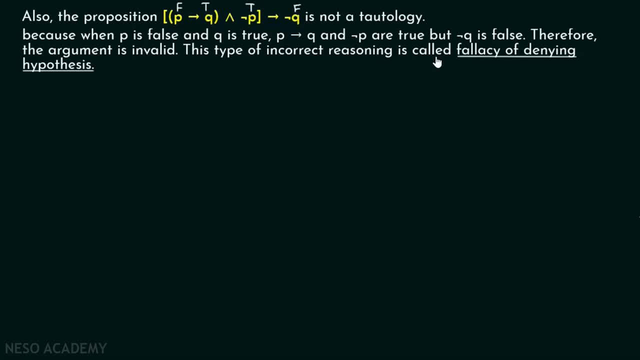 Therefore, the argument is invalid. This type of incorrect reasoning is called fallacy of denying hypothesis. Okay, this is another argument which is a fallacy, And this type of incorrect reasoning is called fallacy of denying hypothesis. Let's consider one more time. 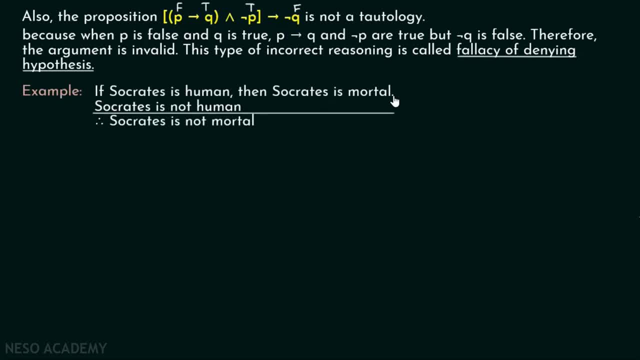 Let's consider one more time. Let's consider one more time. Let's consider one example. If Socrates is human, then Socrates is mortal. Socrates is not human, therefore Socrates is not mortal. Okay, it seems correct, but let's understand this in more details. 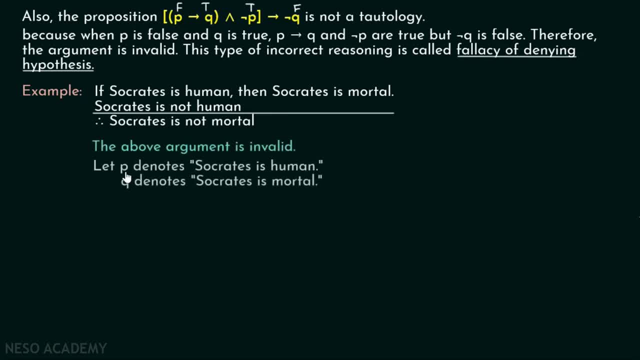 This particular argument is invalid. let me tell you. but why? Let P denote Socrates is human and Q denote Socrates is mortal? Now let's just convert these statements one by one Here: if Socrates is human, then Socrates is mortal. can be represented by: P implies Q. 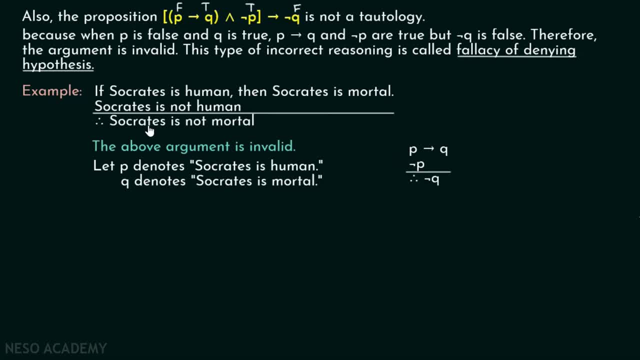 Socrates is not human is represented by Q, Q is represented by not P, and Socrates is not mortal is represented by not Q. It seems like this is a rule of modest tolerance, but it is not. if you closely observe this Here, we know that this is fallacy of denying hypothesis, right. 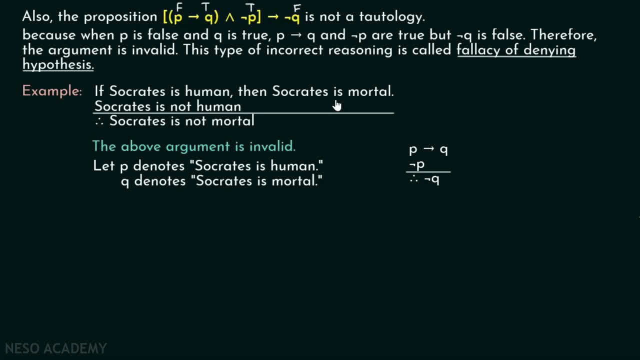 And this is not valid. Okay, if Socrates is human, then Socrates is mortal. Socrates is not human. Can you say that Socrates is not mortal? Obviously not right. If Socrates is not human, then you cannot say that Socrates is not mortal. 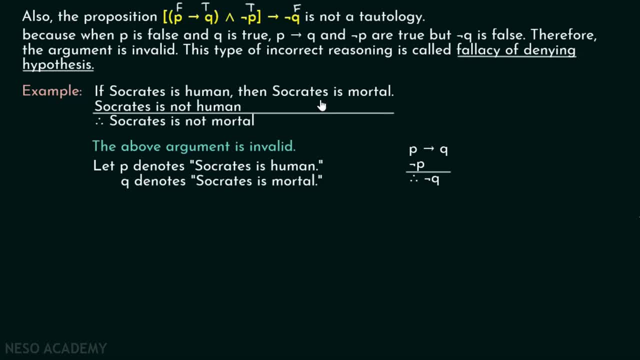 There could be other reasons for Socrates being mortal: mortal, right. So you cannot say that if Socrates is not human, then Socrates is not mortal, But if Socrates is not mortal, then it is clear that Socrates is not human. okay, The other side is. 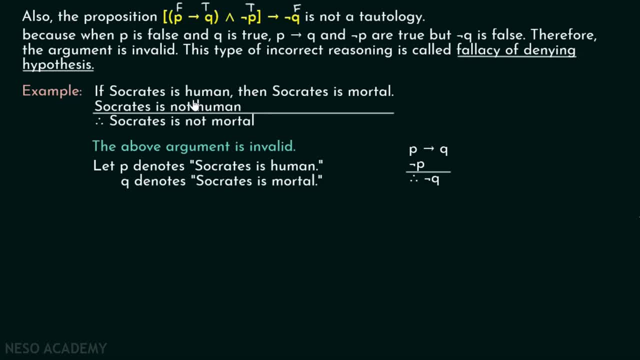 true, fine. So this must be well understood. And now you have understood what is the meaning of fallacy, And we have seen the two different types of arguments, that is, fallacy of affirming the conclusion and fallacy of denying hypothesis. okay, That's it. I'll see you in the next lecture. Thank you.